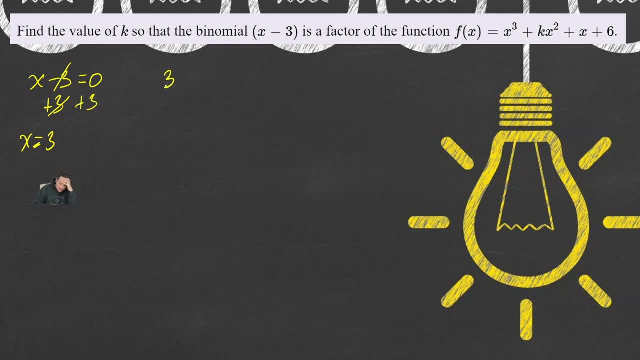 So put u3 over here. That's the root version, So that's why it's positive 3, that's coming from here. And then you set up Synthetic division. so here across the top you're going to put the coefficient. 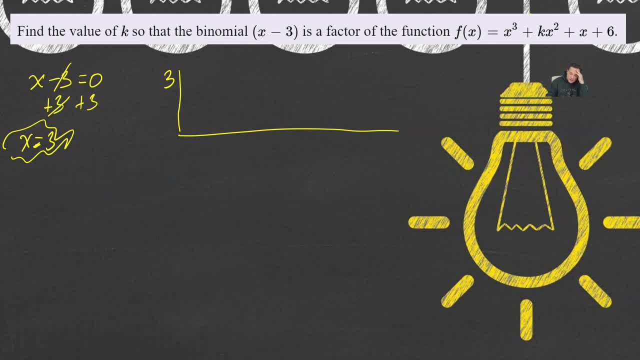 So remember that. up here is the following: right It says x cubed. So the coefficient on the x cubed part that would be equal to 1.. The coefficient on kx squared is just k, so that goes over here. 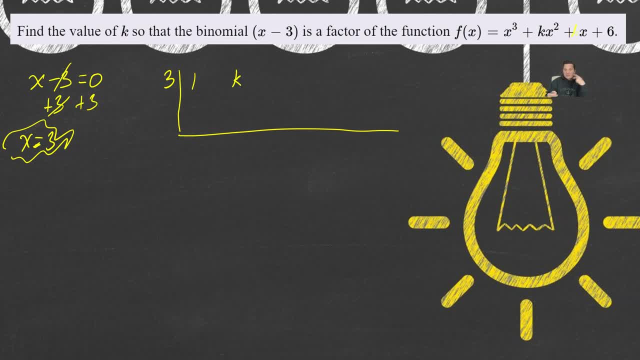 The coefficient on the x term by itself. remember that's like a positive 1 in front of it. so it's 1 over here and the constant is 6.. So you put 6 over here And then you go and you do the process of the synthetic division carefully. 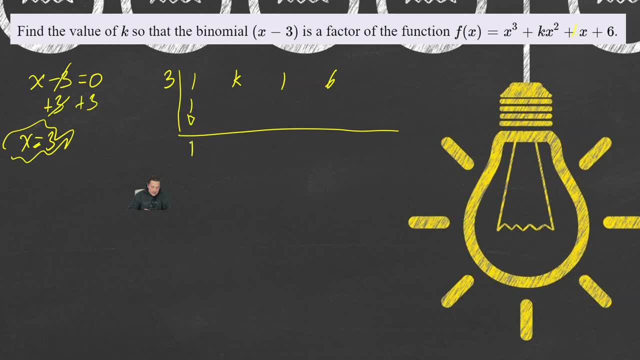 Let's carry that out. First I take this 1 straight down, So it's going to give me net. then 1 times 3, which is 3, that comes down here. And now stop for a second, because above the 3,, as you can see, is a k. 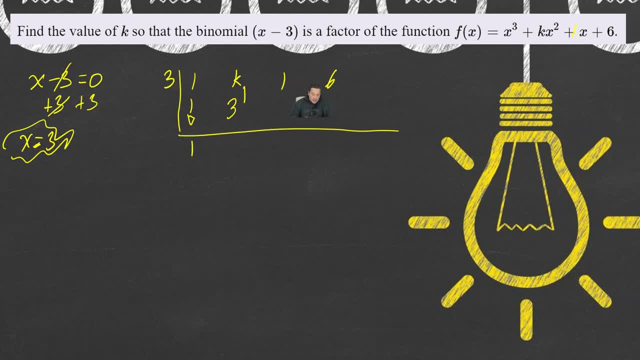 So then you just have to add these straight down, basically this way. okay, So when I do that, it's going to give me the following: k plus 3, which is k plus 3.. Then I continue synthetic division. So when I do that, I'm going to have k plus 3 multiplying the 3, the root. 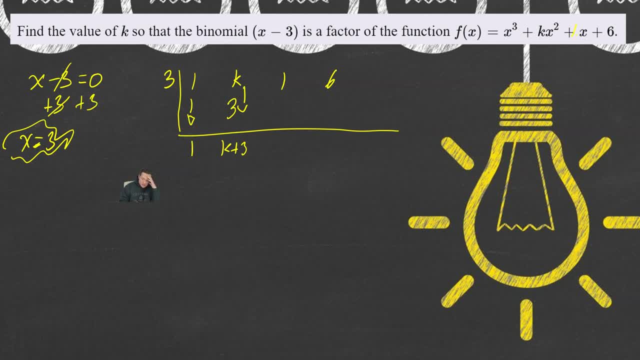 So let's go through this slowly. If you need to, you can make side work out of it. What I mean is the following: I'm going to do 3 times k plus 3.. So when I do that, that's basically 3k plus 9, and that goes over here. 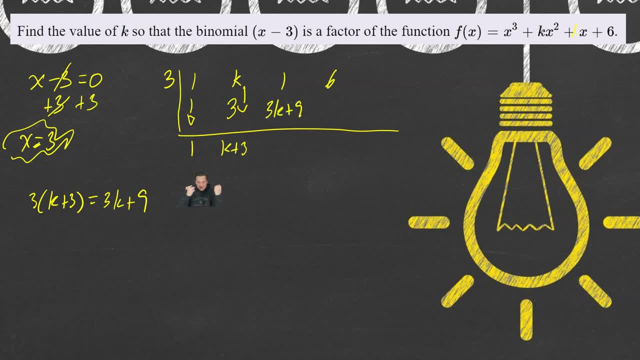 That becomes 3k plus 9, right here. So we're keeping k as a variable here in this process, and then I'm going to add again straight down. So that's going to give me 3k plus 10, because the 3k is one term and the 1 plus the 9 is 10.. 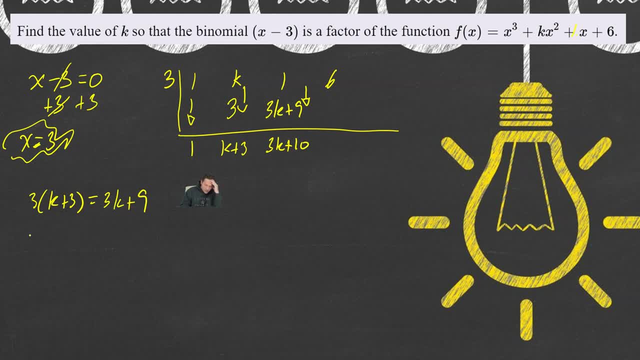 And again I go with the synthetic division process. So I need to do now 3k plus 10, multiplying the 3 on the outside Up here, the root. So when I do that it's going to give me- let's see here, it's going to give me 9k plus 30.. 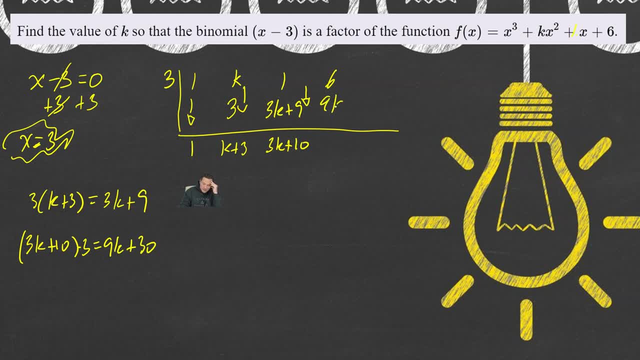 So over here, under the 6, now I'm going to put 9k plus 30. And for the 3 to be a root or the x minus 3 to be a factor, what has to be true is the following: 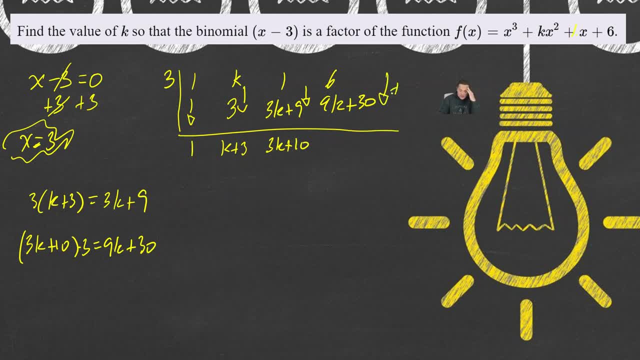 These two things, the 6 and the 9k plus 30 added straight down, have to be equal to 0. In other words, this has to be 0. I'm not saying it is right now. It has to be 0, okay.